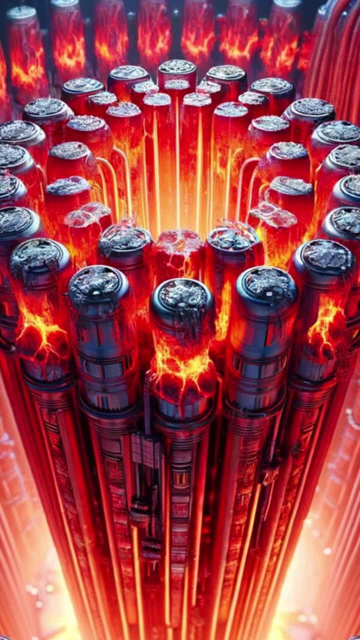 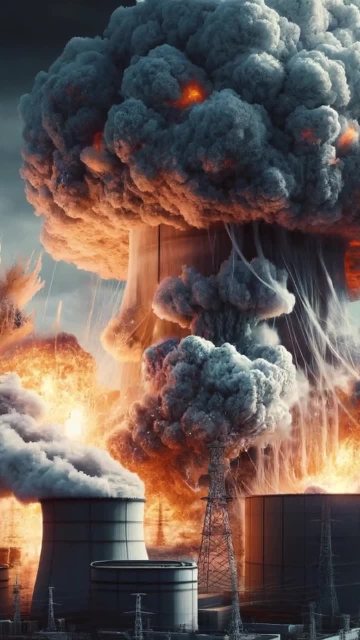 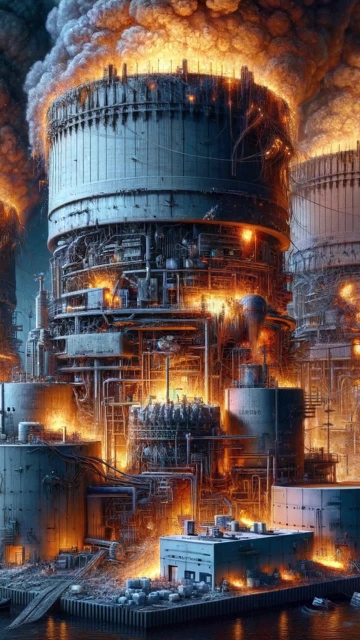 at the Fukushima Daiichi power plant. This loss of cooling led to nuclear fuel overheating and melting, causing hydrogen air explosions and releasing radioactive material. Backup diesel generators intended to provide power for cooling systems were flooded by the tsunami. Without adequate cooling, the reactors' temperatures rose, leading to meltdowns in. 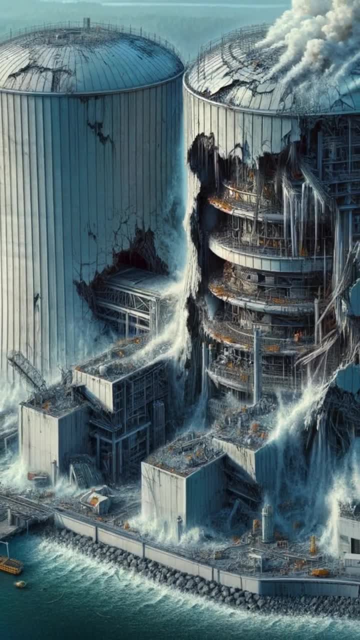 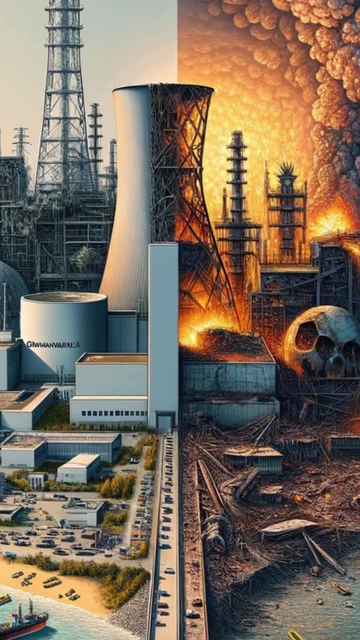 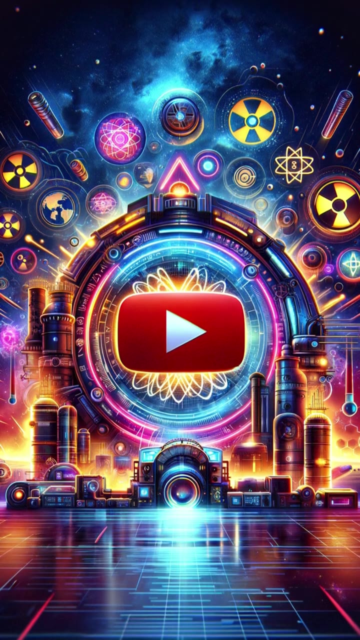 reactors 1,, 2, and 3.. Containment structures were damaged and large amounts of radioactive material were released into the environment, making this the most severe nuclear accident since the Chernobyl disaster in 1986.. Now, if you enjoyed this video, subscribe for more.